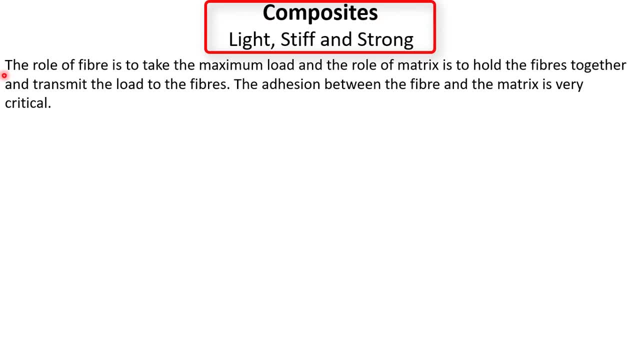 combination of two or more than two phases. One is the matrix and another is the filler, which comes in the form of fibers or particulates and so on. The role of fiber is to take the maximum load and the role of matrix is to hold the fibers together and transmit the load to the 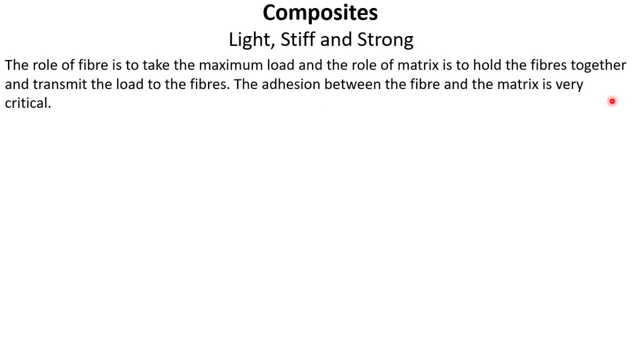 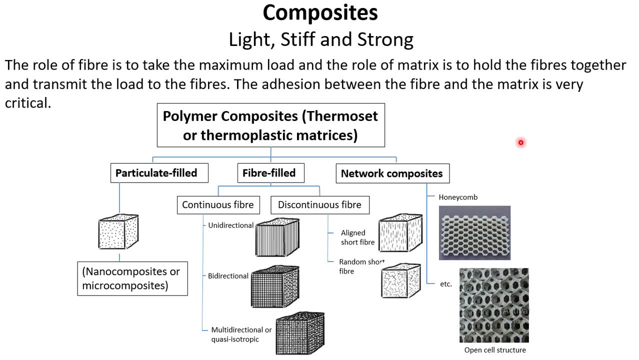 fibers. The adhesion between the fiber and the matrix is very critical in this case. These are the classifications of polymer composites. They can be made of thermoset or thermoplastic matrices. Polymer composites can be divided into two or more than two phases. Polymer composites can be divided into two or more than two phases. 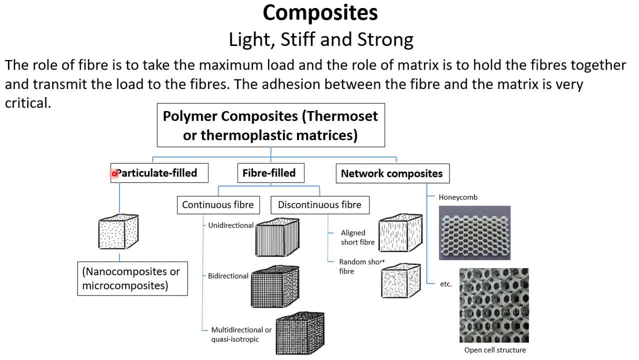 Polymer composites can be divided into two or more than two phases. Polymer composites can be divided into three major classes. One is called particulate filled, another is fiber filled and the third one is network composites. The particulate filled composite materials have fillers, but they are in the form of particles. 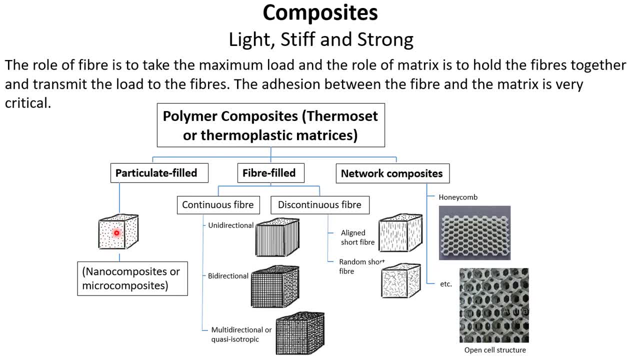 not long fibers. The size of these particles can be from micron to nano range and therefore we have got two types of particulate: filled composites: Nano composites or micro composites. This are basically defined by the size of the particle themselves, that is, the diameter of the particles. 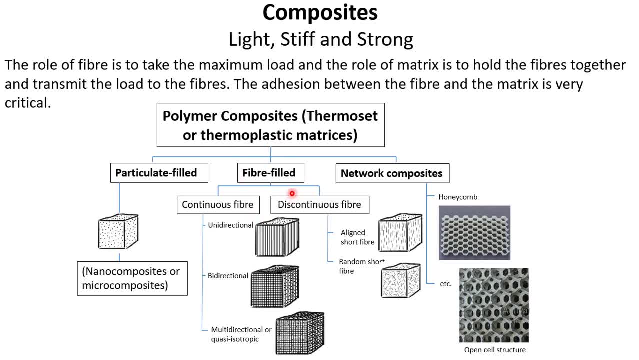 The second class, which are the fiber filled, are the most used composites. They are of two types. One is of continuous fiber and another is discontinuous fiber. The continuous fiber, as the name suggests. here the fibers are very long and they continuously go along the length of the 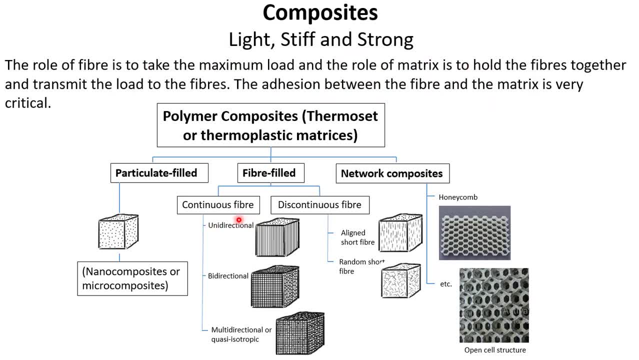 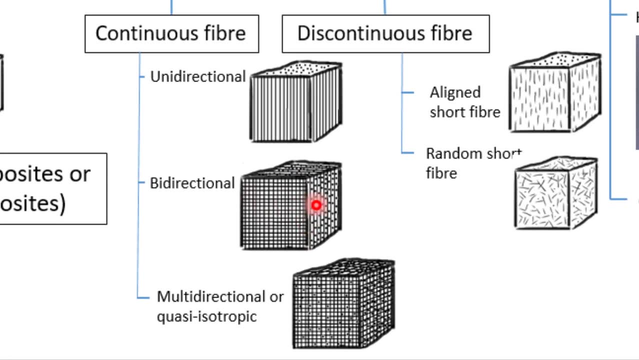 part. They can be of three types. unidirectional, that means the fibers are all in one direction, So here, in this case, they are all in this length direction. It can be bidirectional, so in this case some fibers are in this vertical direction and some fibers are. 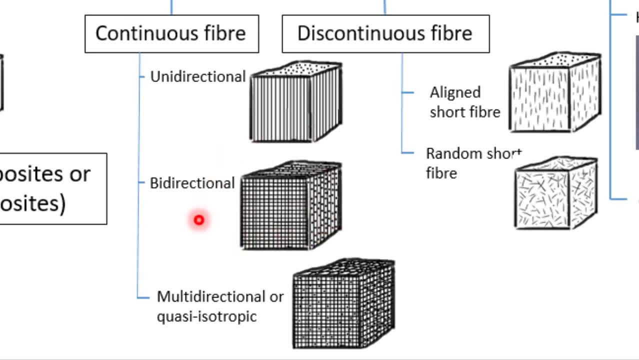 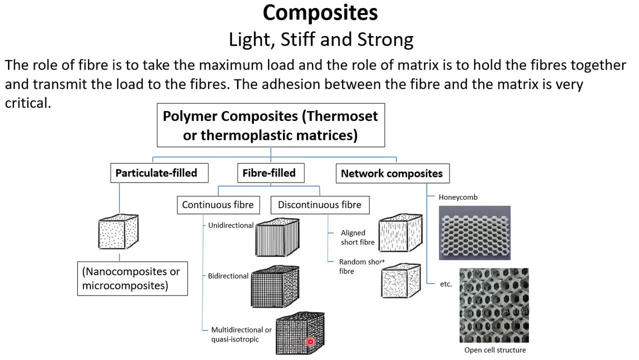 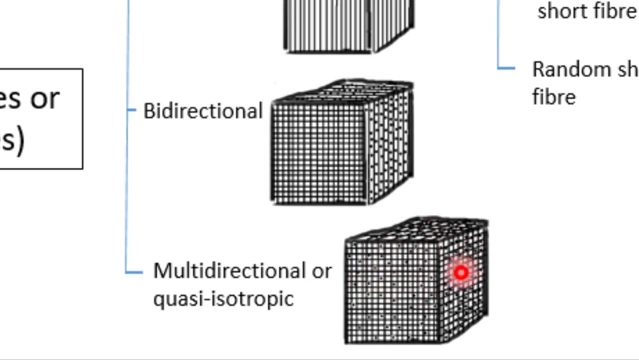 in this horizontal direction, So only two directions are used, and it can be also multi-directional or quasi isotropic. So in multi-directional the fibers are in more than two directions. So either they can be three distinct directions or they can be more than three directions and they produce. 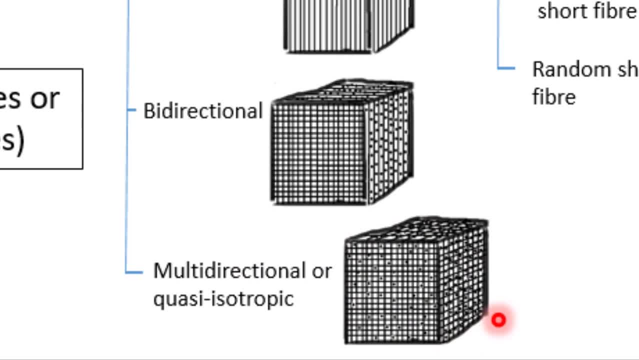 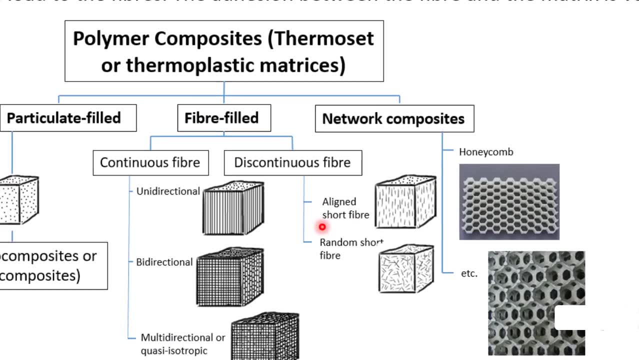 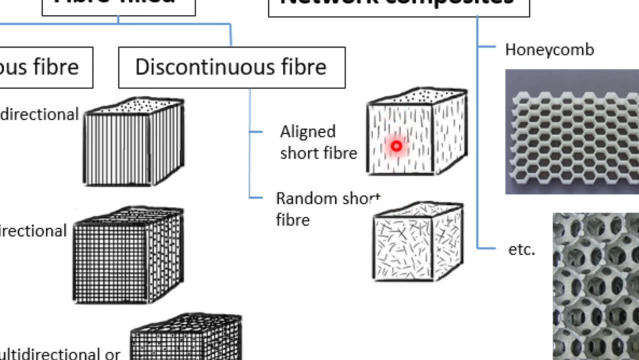 what is called quasi isotropic. So these kind of composites have very homogeneous type of properties. Within fiber field there are discontinuous fibers. So these kind of composites have fibers, but these fibers are not not continuous, but rather they are chopped. They are also known as chopped fiber. 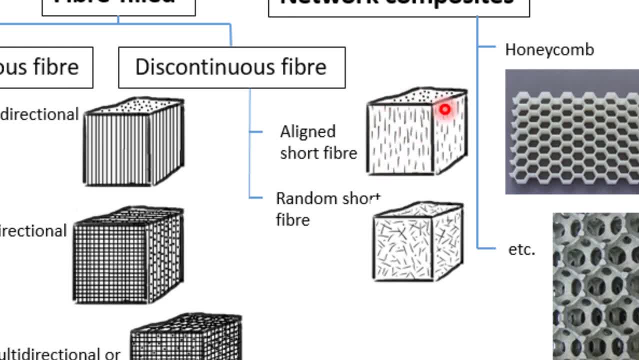 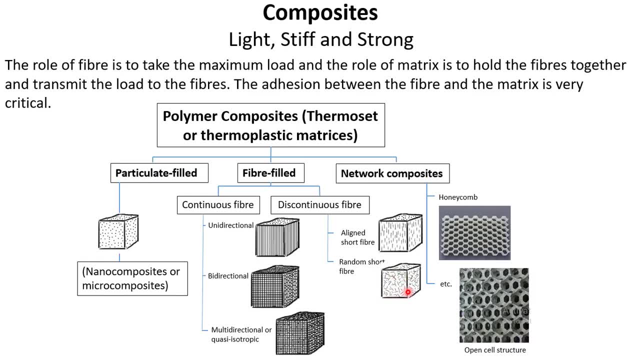 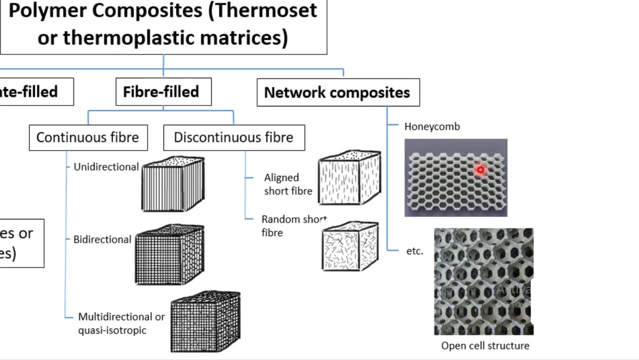 composites. So in some cases these chopped fibers can be aligned in one direction Or they can be at random, So in this case they are at random in all directions possible. The third class of polymer composites are network composites, So in this case the filler is in the 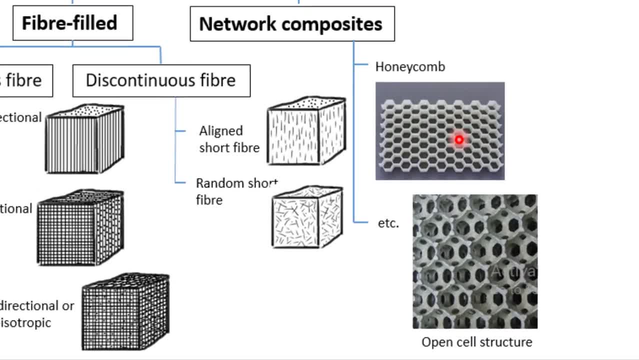 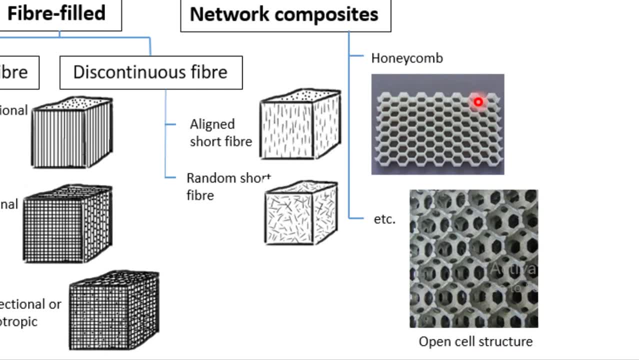 form of some sort of network or some sort of structure. So, for example, we have honeycomb structure here and this one is open cell structure. So the filler material can be in the form of these cell structures and they can be filled with. the empty spaces can be filled. 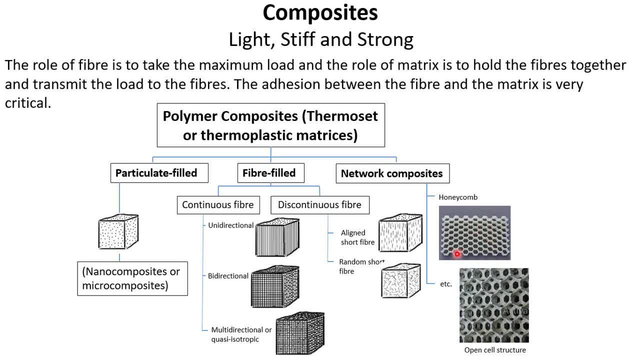 with the matrix or any kind of polymer, So this will also produce a composite material, But in our case mostly we will be talking about continuous or discontinuous fiber composites or particulate composites, Typical fibers and their tensile properties, Although there are many. 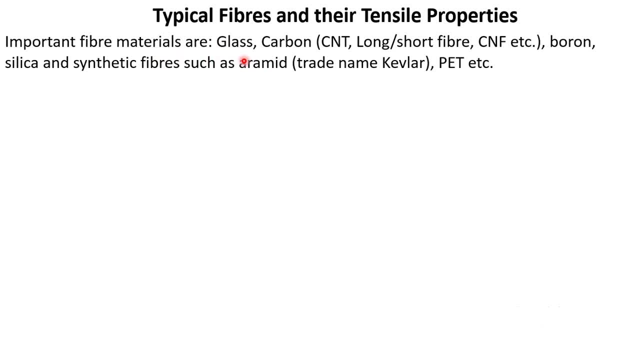 different types of fibers we can use, but these are the typical fibers that we use for making polymer composites. Glass fiber was the earliest one, So the very first fiber reinforced plastics were made of glass. Carbon fiber came along later on In the carbon material. there are different types of fibers. 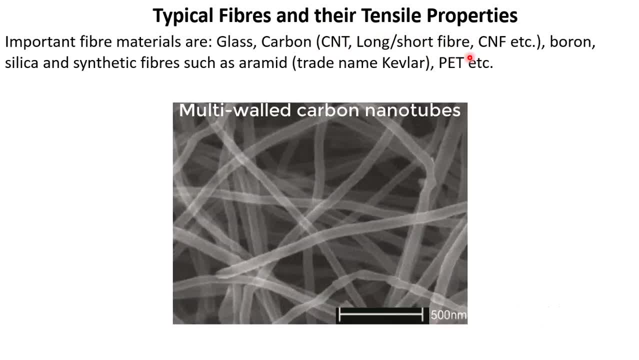 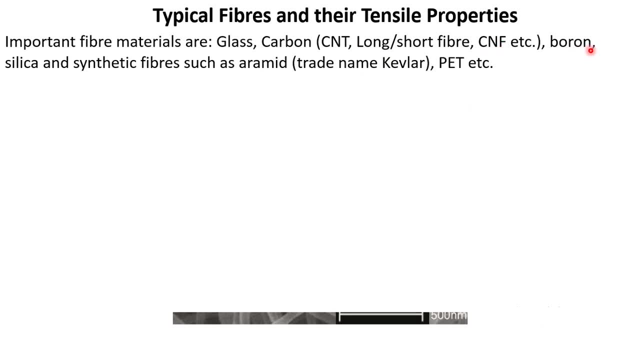 So, for example, carbon nanotube, long or short carbon fibers, carbon nanofiber, etc. So there are different types of carbon material we can use in the composites. Boron can be used in the form of fiber, Silica or even synthetic fibers such as aramid can be used. 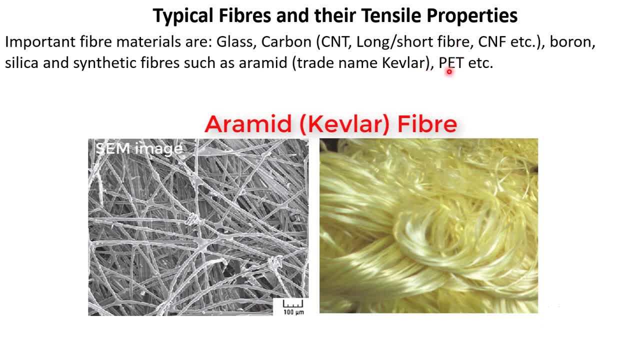 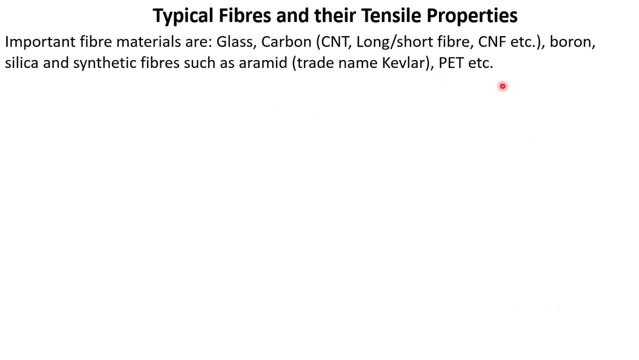 which is also known as Kevlar. Even PET fiber can also be used, So there are many different types of fibers. One of the important aspect of these fibers is that these fibers are extremely strong compared to the matrix. Here we have got stress and strength curves for many of these fibers. 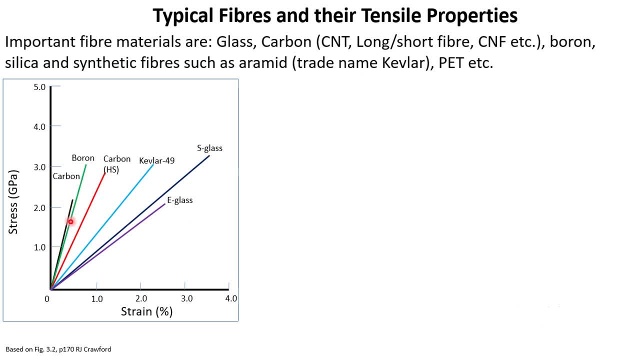 we have just explained. For example, carbon is here. Next is boron, another type of carbon fiber. Kevlar Glass has got two types: S and E type. here We can see that carbon and boron gives the highest stiffness because the value of these personality fibers. makes performance of the carbon fiber more positive as compared to other types of fibers. You can see these fibers together. The transfer points can be defined in terms of theends问题 and different types of fibers depending on the day and time of the moment. So, as we can see that carbonly respond books. there are a few different types of fibers in меня and one of the most common is carbon sugar In many. all of them have various colored fibers. They are a type of pounds. 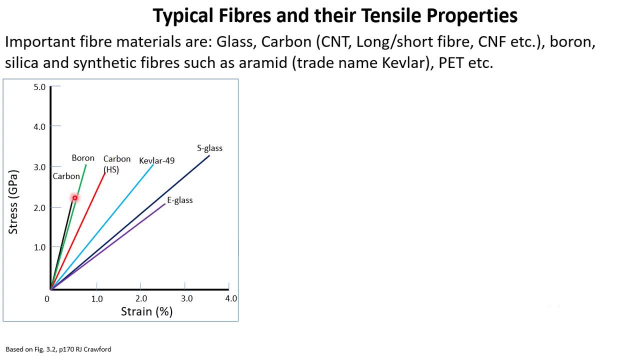 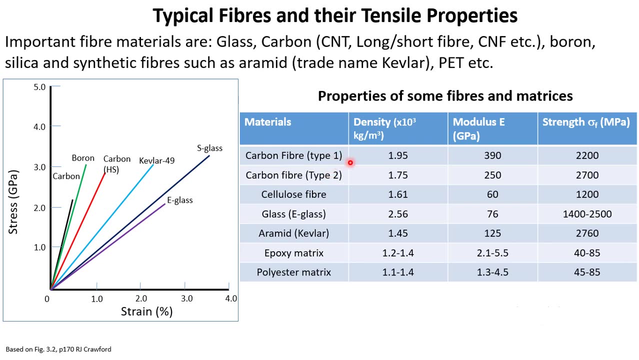 because the value of E or Young's modulus is high for this carbon and boron fiber, whereas glass fiber gives the lowest value of elastic modulus. So now we can look at the data themselves. So carbon fiber another. there are two types of carbon fiber: type 1 and type 2.. Cellulose fiber is 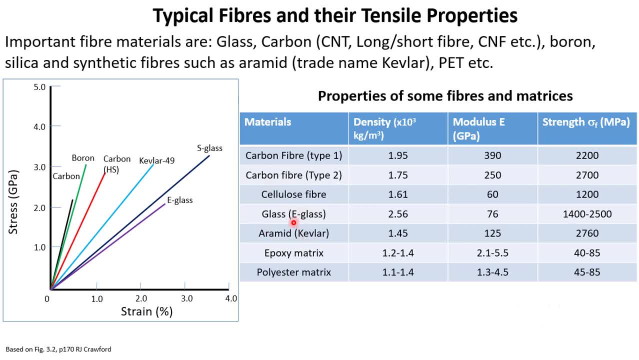 what we can obtain from wood, glass fiber, aramid, epoxy matrix. So these, these two are the matrices, epoxy and polyester. We can see that the density wise glass fiber is the denser. So this has got density of 2.56 multiplied by 10 to the power cube kg per meter cube. So glass fiber makes 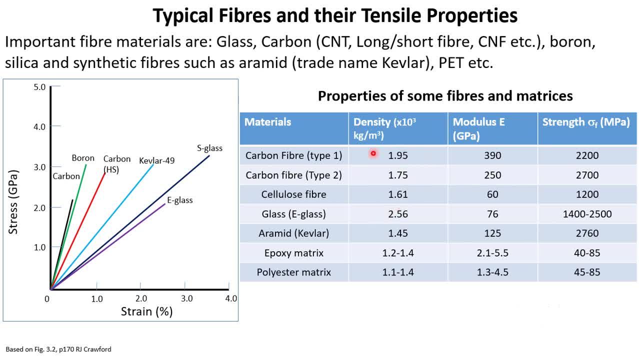 the heaviest composite, whereas other fibers are more or less very similar in values. The modulus we can see carbon fiber has the highest modulus here, followed by aramid fiber. Glass fiber do not give very high value of modulus, So in terms of stiffness, 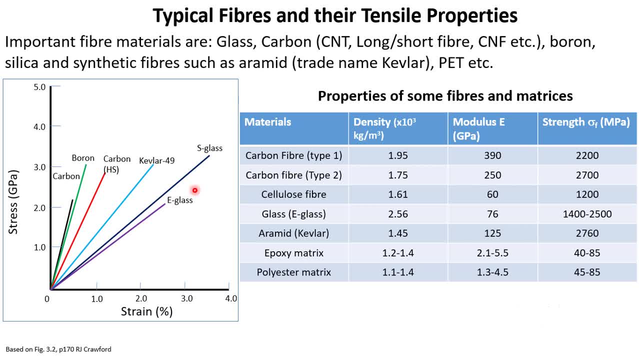 as we saw in this graph, stiffness is not very high for glass fiber. Boron is almost close to the carbon fiber In terms of strength. we can see that carbon fiber has very high strength, but aramid fiber also gives a very, very high strength, So aramid fiber does not have very. 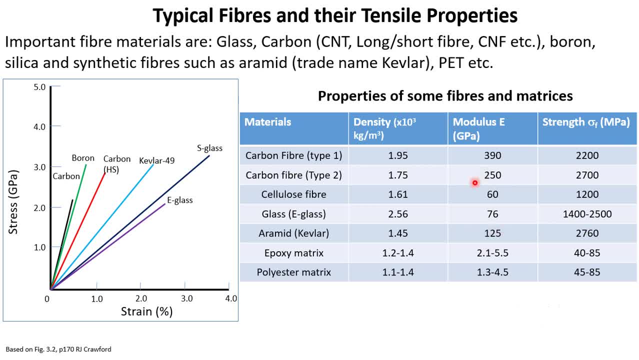 high modulus. but modulus is in between carbon and glass fiber, but strength wise aramid fiber fiber is comparable to carbon fiber and these two are epoxy and polyester matrices. so the role of the matrix is basically to hold the fiber together, but there are many other properties that are. 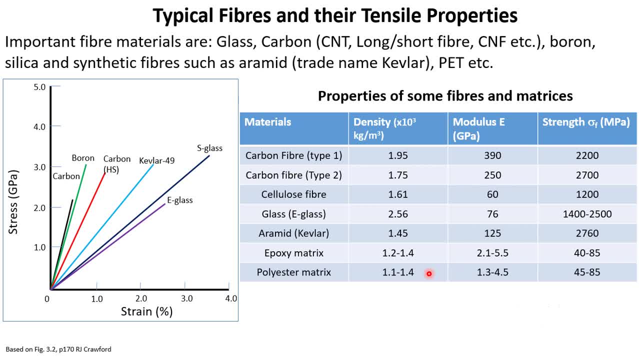 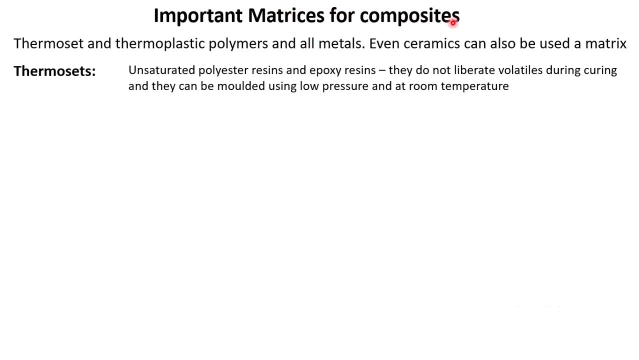 important in order for us to get the best matrix for the composites. these pictures show the three main fibers. this is the glass fiber, how it looks, the carbon fiber and this is the aramid fiber. now let let's look at important matrices for composites, both thermoset and thermoplastics. 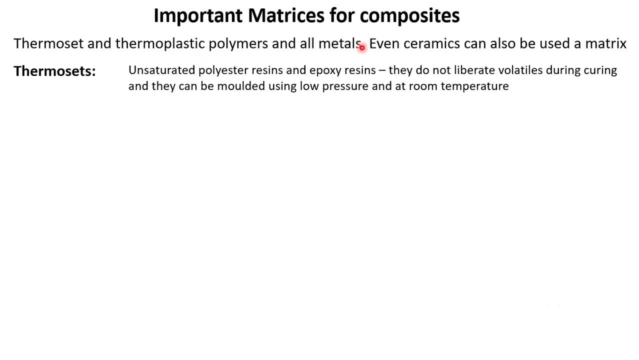 can be used for making matrices. even metals can also be used for making matrices, but here we are mostly talking about polymer based composites, thermosets, unsaturated polyester resins and epoxy resins. they are used very commonly. they do not liberate volatiles during curing and 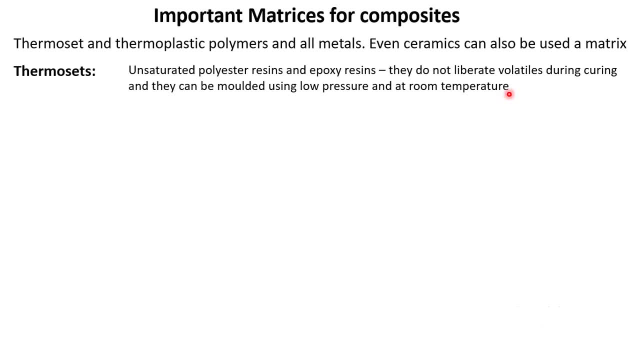 they can be molded using low pressure and room temperature. so this is very, very important. if epoxy or if the matrix polymer releases volatile materials or like volatile gases during curing process, so that will introduce lots of defects in terms of bubbles. so those defects are not desired in composites. so that's why we select polyester and epoxy resins also. these two resins can be 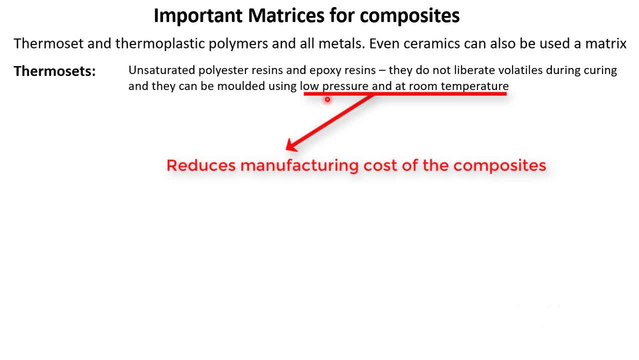 molded at low pressure, that means this normal atmospheric pressure, and at room temperature. so even at room temperature it can be molded at low pressure, so that means this normal atmospheric pressure, and at room temperature. so even at room temperature they can cure. you can initiate the curing process by adding hardener. so these properties of epoxy and 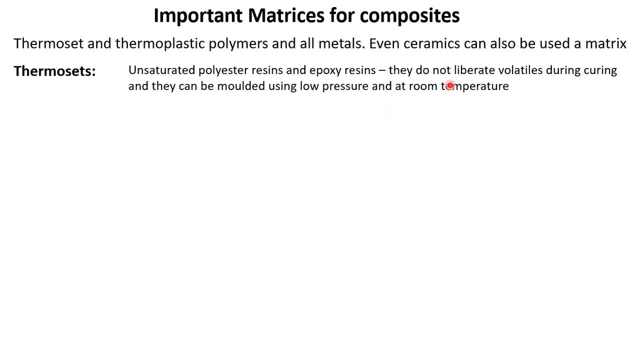 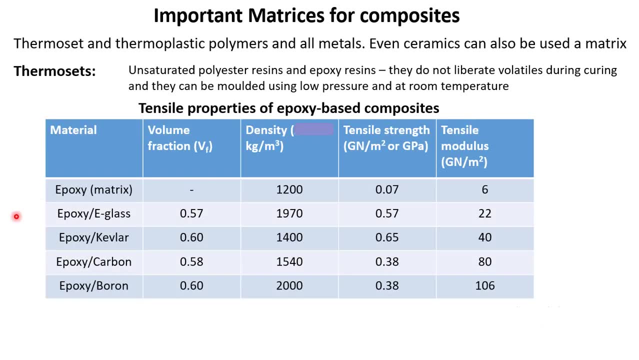 polyester resins give much of advantage compared to other thermosets. tensile properties of epoxy-based composites. so let's look at some epoxy-based composites. so, for example, this is the matrix. matrix is the epoxy with glass fiber, kevlar fiber, carbon and boron and we have got volume fraction. 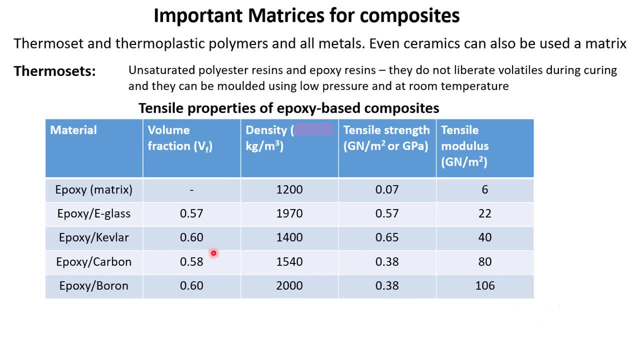 which is close 57 to 50 degrees celsius. so this is the matrix, matrix is the epoxy with glass, fiber, kevlar, fiber, carbon and boron, and we have got volume fraction which is close 57 to 50 degrees celsius: zero point five seven, zero point six, zero point five eight, zero point six. so 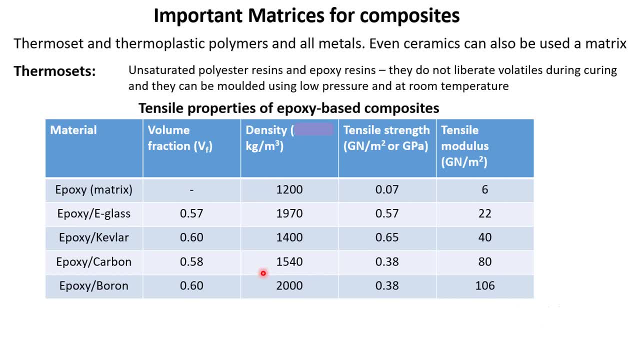 very close to each other and we have got the density of these composite materials. so epoxy is a light material and when we add glass fiber the density increases. so density of boron fiber composite is the highest, followed by epoxy, which is very close to boron in terms of density. and 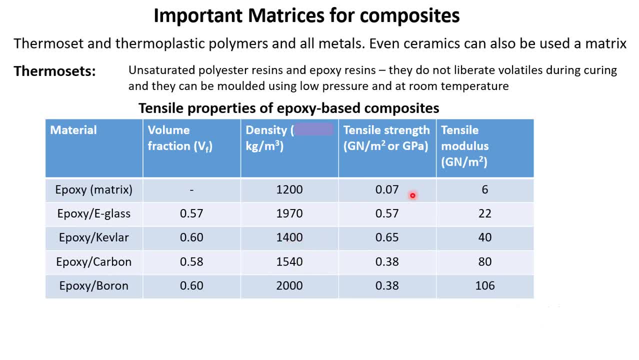 then comes carbon and kevlar. when we look at the tensile strength, of course, the tensile strength of epoxy is very, very low: 0.07 gigapascal. after adding these fibers we see that the tensile strength has improved. in the case of glass fiber, the tensile strength is 0.57. so this tensile 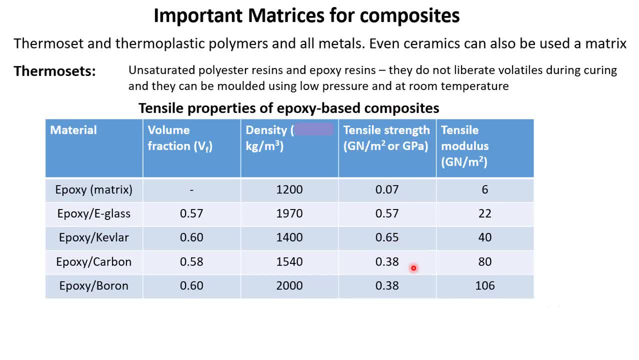 strength is actually the fracture strength for kevlar 0.65, for carbon 0.38 and for boron 0.38. in terms of modulus, we can see that epoxy with glass fiber has got modulus which is the lowest highest modulus we can obtain from boron, followed by carbon and kevlar. so these are some typical data. 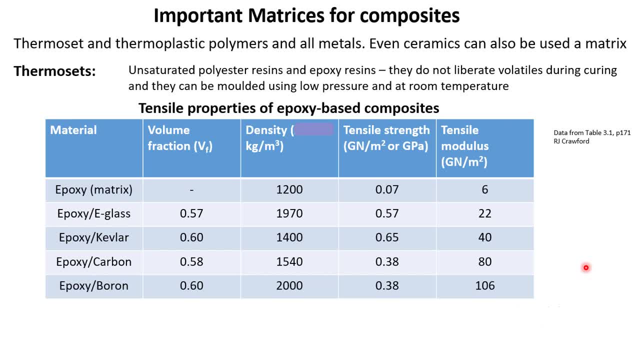 taken from some references in different literature. you will find these values are slightly different. so, depending upon the how the experiments are conducted, we can find the data might vary to some extent, but these are the typical type of data we will obtain in experiments. so we can say that thermosets provide high strength. 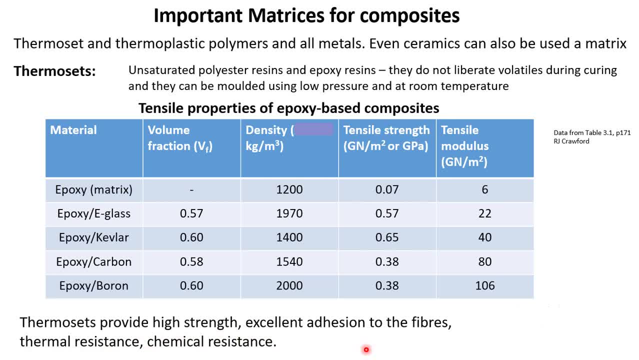 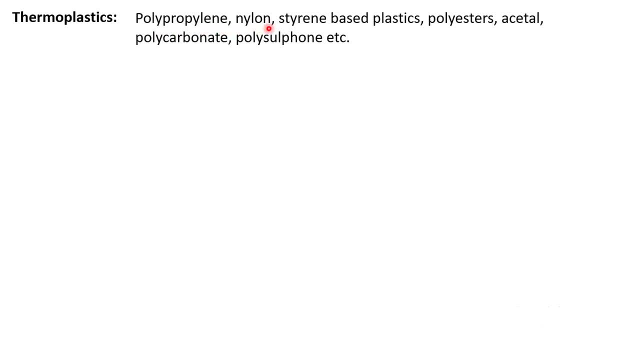 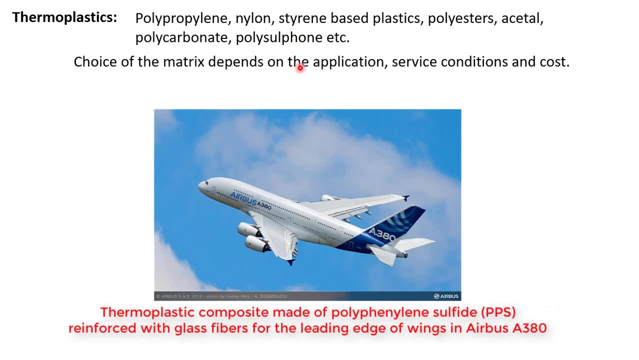 excellent addition to the fibers. thermal resistance and chemical resistance. thermoplastics can also be used as the matrix. so common thermoplastics are polypropylene, nylon, styrene based plastics, polyesters, acetyl, polycarbonate, polysulfone, etc. so choice of the matrix depends. 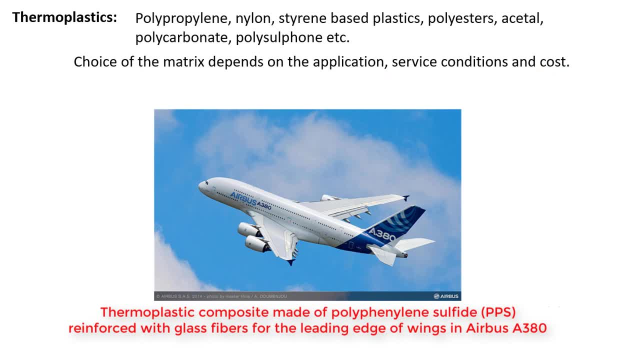 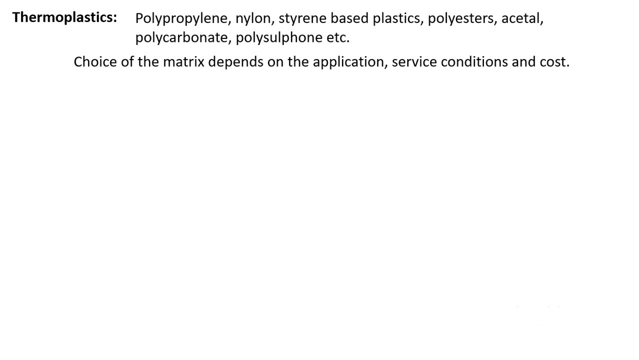 on the application, service conditions and cost. so application and service conditions are very important. so the review of the application of thermoplastics, as we said, is very important. for example, temperature will be the guiding factor in selecting some of the matrix materials. similarly, cost is also an important factor if the application 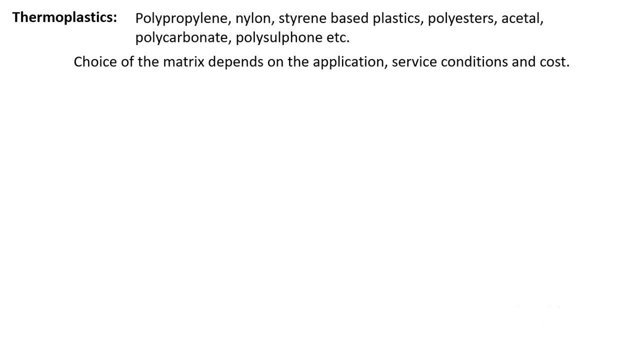 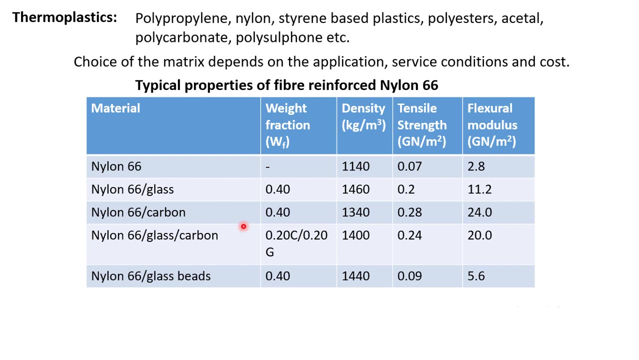 if the cost has to be low. in that case we will have to go for a plastic which is low in cost. typical properties of fiber: reinforced nylon 66. so nylon is a thermoplastic material. here you can see that we have different percentages of fiber in the range of 0.4 glass fiber, 0.4 with carbon glass and carbon fiber. 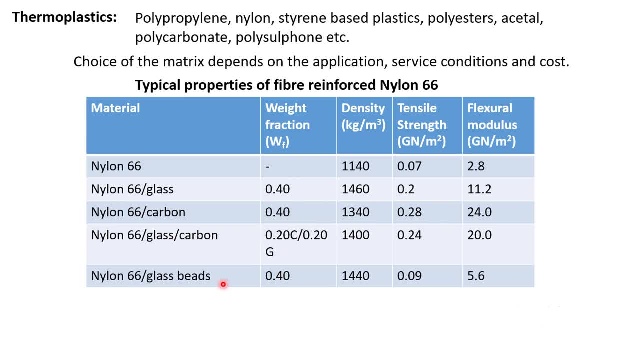 together 0.2 and 0.2 and glass beads. so these are not fiber, these are beads 0.4. this is the weight fraction. now we have got the density values and we can look at the tensile strength. so this, this is gigapascal. so nylon tensile strength is very close to what we can get for 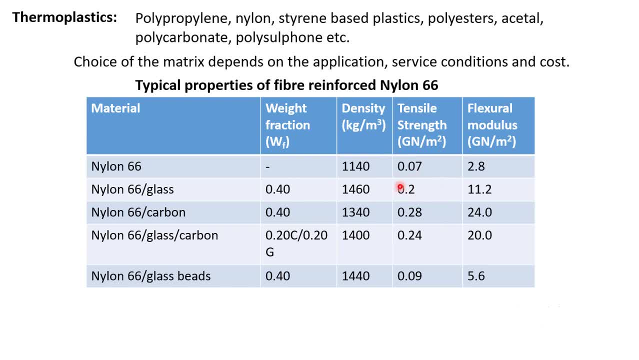 epoxy 0.07, gigapascal, and this composite has got 0.2, with carbon fiber 0.28. with glass and carbon fiber 0.24, so it comes somewhere in between these two. and with glass beads we can get 0.09, so we can see that glass beads do not. 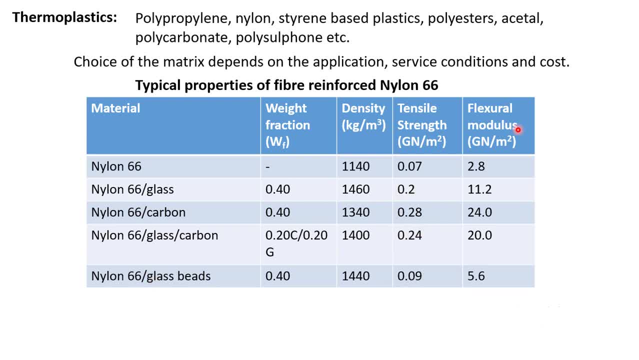 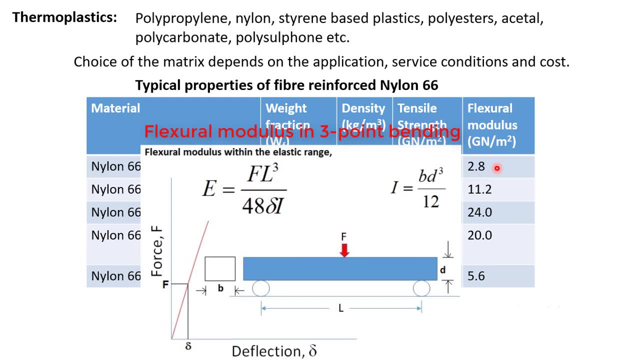 change confident than iron. it sailors very well. we have used a full load of a given Cou roster which we will also be using under water as it consistent. so for the total weight of the vessels, what we are adding is 0.03kg for brass beads. 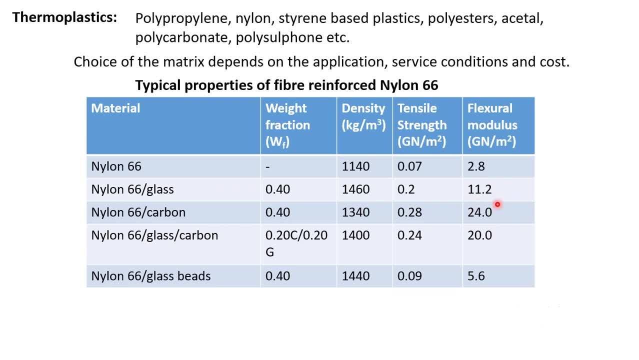 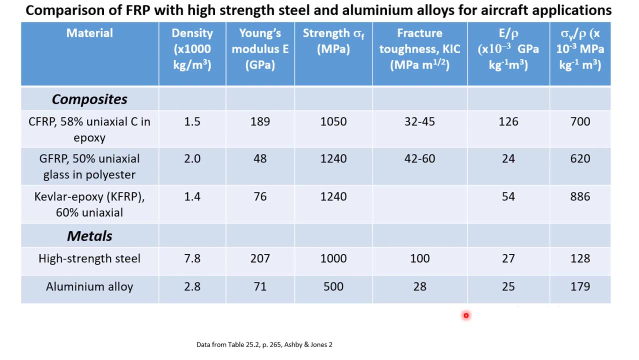 so that is irregular. plus the maximum weight of the vessel, this is what we have. we are here going to apply theillaων 0, .4 mm. 6 milliliter from couple Murphy's. In this slide we will compare mechanical properties of composites with those of metals. 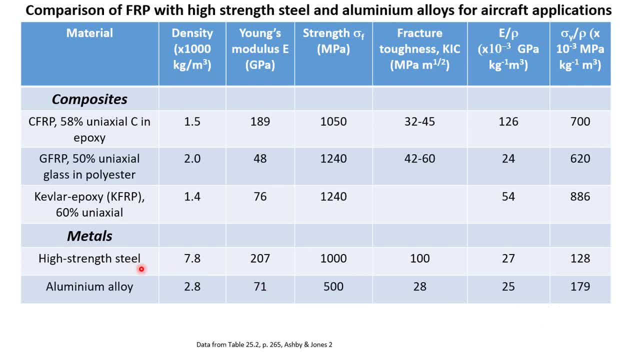 Some of the metals that we use for high-end applications, such as high-strength steel and aluminum alloy. These two types of metals are actually used for many parts in aircrafts. In composites we have carbon fiber, reinforced plastics, 58% uniaxial carbon in epoxy. 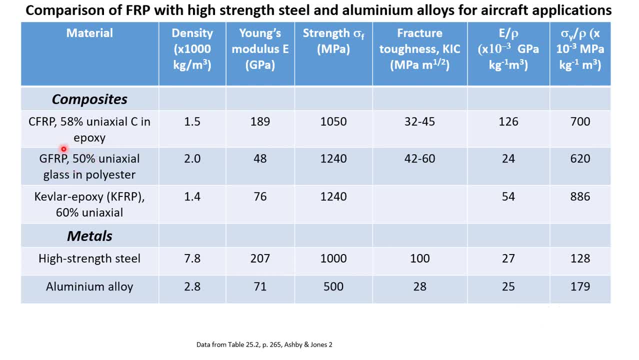 The second one is glass fiber reinforced plastics. This is 50% uniaxial glass in polyester, So these matrices are different. Then we have Kevlar with epoxy- KFRP, 60% uniaxial. So these two composites, Kevlar, epoxy and CFRP, are very similar in percentage. 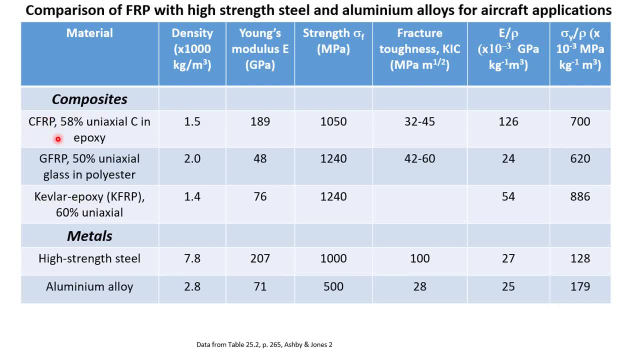 We do not have the data whether these are volume percent or these are weight percent, But most probably these are in weight percent And this one is glass fiber with polyester. So the matrix is different. In this case it is not epoxy. So let us compare the mechanical properties, starting with first we will compare the density. 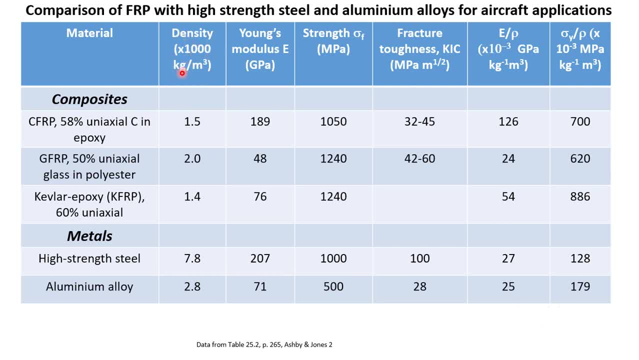 So density units are here multiplied by 1000 kg per meter cube. So here we can see that GFRP is the heaviest among these three composites, Whereas CFRP is 1.5 and Kevlar epoxy composite is 1.4.. 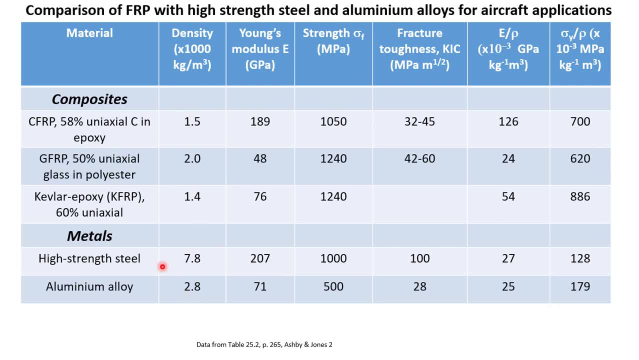 Compared to these three composites, the metals are much more heavier because their density is high. Aluminium is considered as light metal and steel has got density in the range of 7.8. here Now we will compare the modulus Young's modulus in gigapascal. 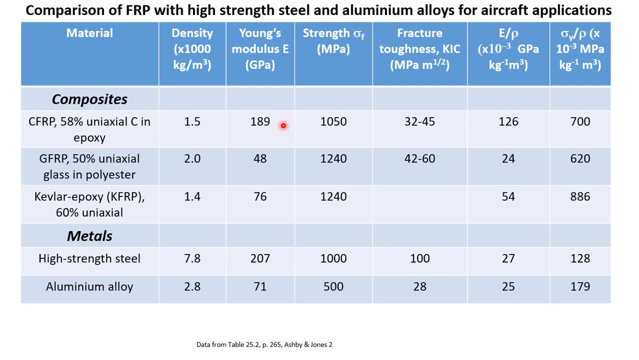 So CFRP gives a very high value of Young's modulus And Kevlar is considered as light metal. Young's modulus is 189.. So this is the stiffest material among these three composites And we can compare 189 with high strength steels, almost close to high strength steel. 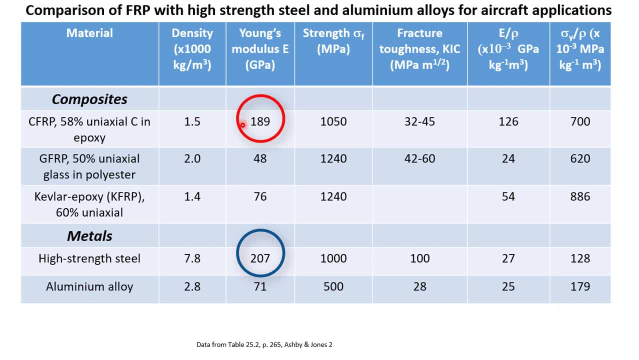 Steel is considered as a very stiff material, So CFRP can provide stiffness very close to high strength steel. Aluminium alloy has lower stiffness, which is comparable to the stiffness of Kevlar epoxy. composite GFRP has got very low Young's modulus. 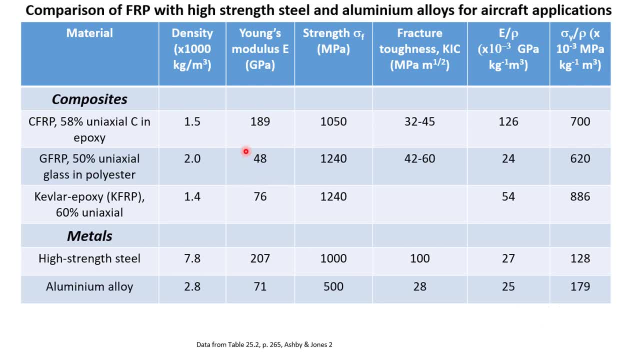 So therefore it is not as stiff. Now, looking at the strength among composites, CFRP is slightly lower compared to Kevlar. Both have epoxy as the matrix, So Kevlar is better in terms of strength And here GFRP has got higher strength. 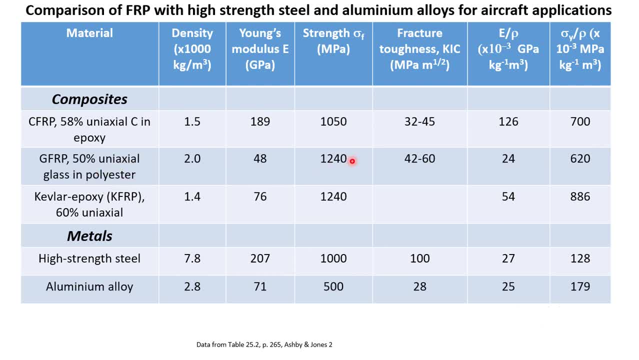 And because in this case the matrix is different And also we should know that the properties of the fibers may vary from manufacturer to manufacturer. Similarly, the properties of the matrix also may vary depending upon the process. So therefore we cannot always compare very precisely. 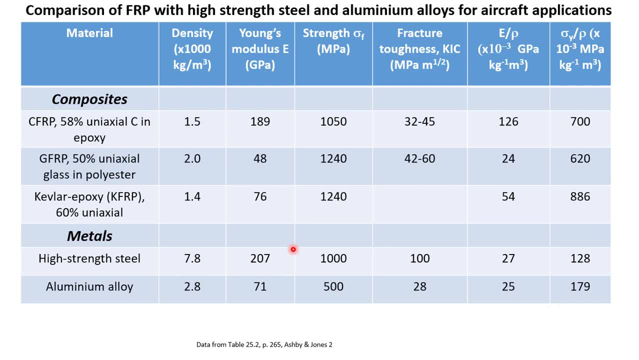 But these are typical values and good for comparison. Compared to composites, metals have lower strength. So high strength steel, which is considered a very high strength material, has 1000 MPa, whereas aluminum is very low. Now we will compare fracture toughness. 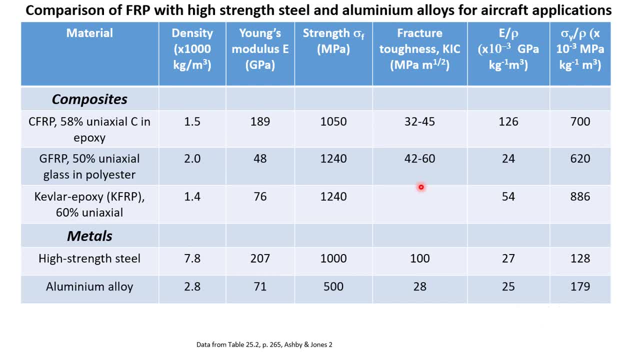 Because fracture toughness, along with modulus and strength, is a very important mechanical property. If the material has very high strength but low in fracture toughness, then this material may not be used for very specialized applications. So here we see that CFRP has got fracture toughness of, in this units MPa to the power. 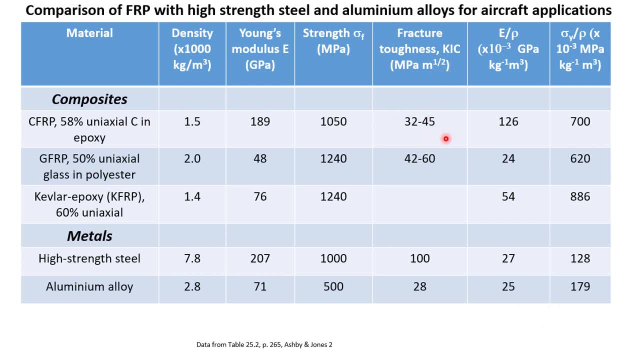 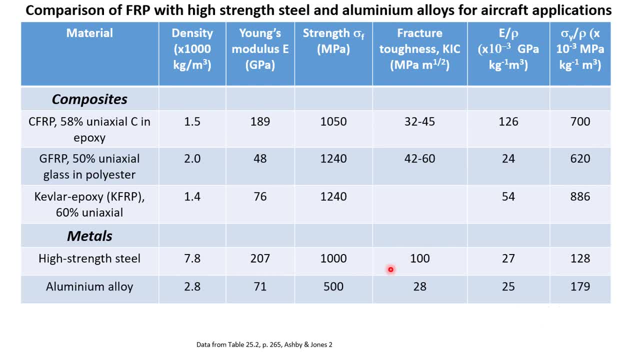 And GFRP with polyester matrix has slightly better fracture toughness. Steel… high strength steel has very high fracture toughness, whereas aluminum is on the lower side. So here we can see that these two composites give fairly good fracture toughness, but not as good as steel. 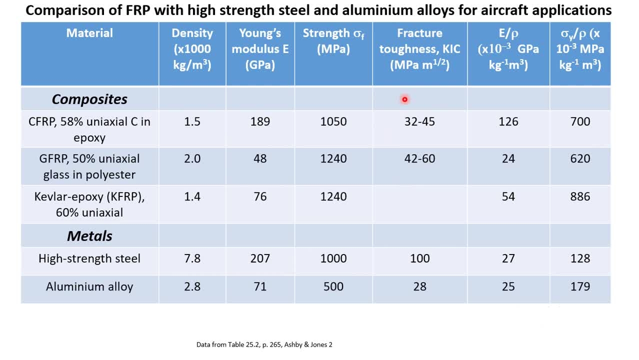 And we know that these materials will not fail in a ductile manner. but their fracture mechanism is different and that gives rise to a higher fracture toughness, And we will talk about the mechanism of fracture toughness in a future video in which I will discuss these two structures. 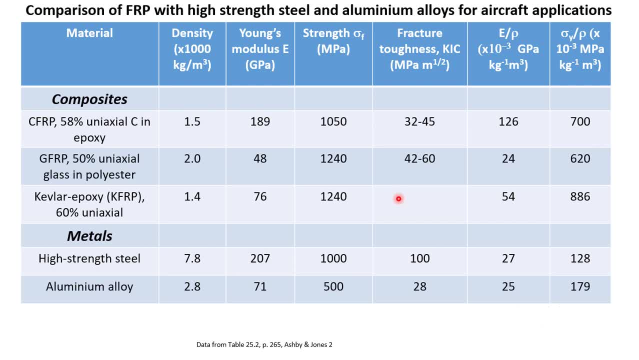 toughness in another video. We do not have data for Kevlar epoxy, but Kevlar is also considered as a very tough fiber and therefore I expect that Kevlar epoxy will have good in the similar range fracture toughness. So comparing these mechanical properties, we can see that, in terms of stiffness, carbon fiber. 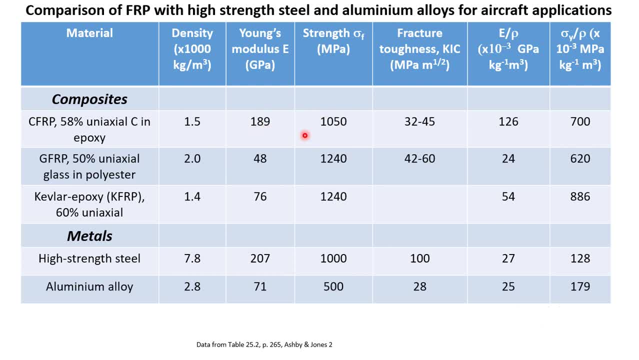 reinforced plastics are good In terms of strength. all of these composites have very good value compared to the metals and in terms of toughness, although steel is very good. but these polymers also give quite good values. Now we will compare two more parameters. The first one is E over Rho. E is the modulus. 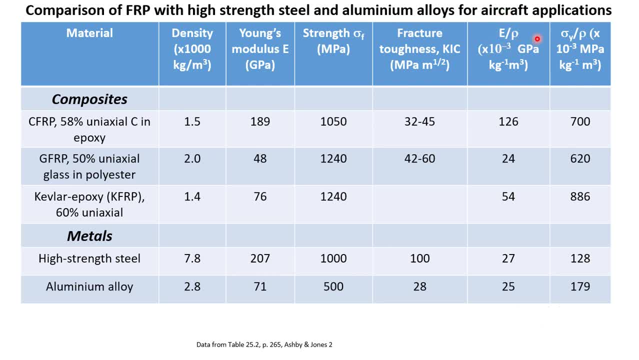 tensile modulus and Rho is the density. So E over Rho ratio basically tells us how much is the modulus per unit density. So for each material we will compare E over Rho over rho and this value: the higher the ratio, lighter the material will be for its stiffness. 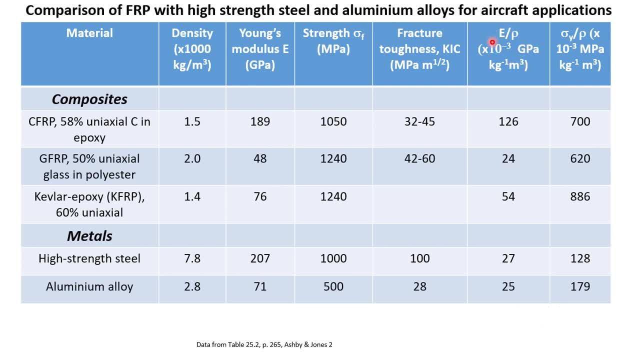 that means that material will be light but stiff. So if we compare these using the same units here, CFRP gives extremely high value of e over rho ratio 126.. So from this point of view we can say that CFRP is a very stiff material for its density. that means you can make a structure. 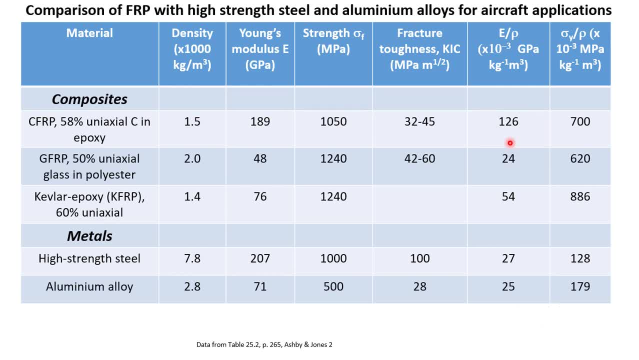 very light but very stiff. Compare CFRP with steel. Steel has got very low value of e over rho ratio, which means that steel, although you can get a very stiff structure but the weight will be the price to pay, means it will be very heavy. Other composites- glass fiber, reinforced composite- is not 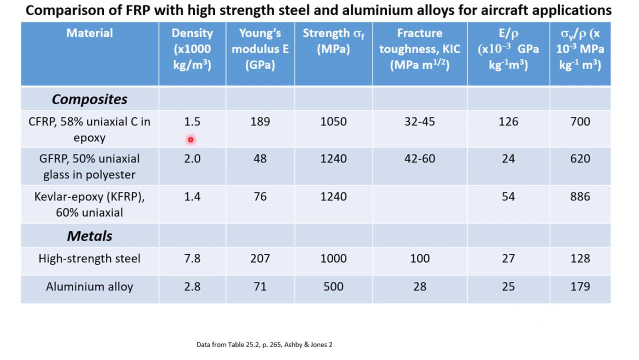 very good in that sense because density is high for this material and also the stiffness is is quite low, in fact lowest among all the materials here. So therefore, glass fiber reinforced composite will not be considered as a light material, stiff and light material, and that's the reason why glass fiber composites. 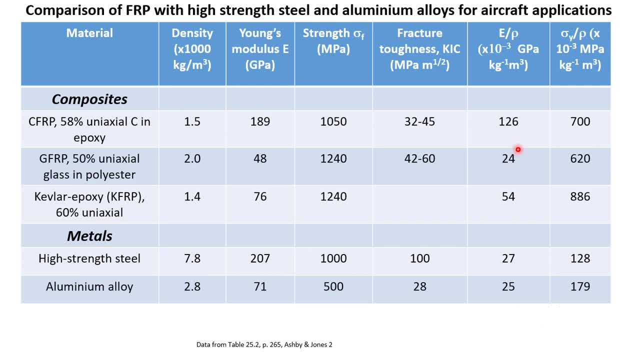 are not used for aircraft applications. Kevlar composites also give quite good value. 54, which is much larger than these two metals. So from the stiffness and lightness point of view we can say that CFRP is the best. second will be KFRP. Now another ratio. 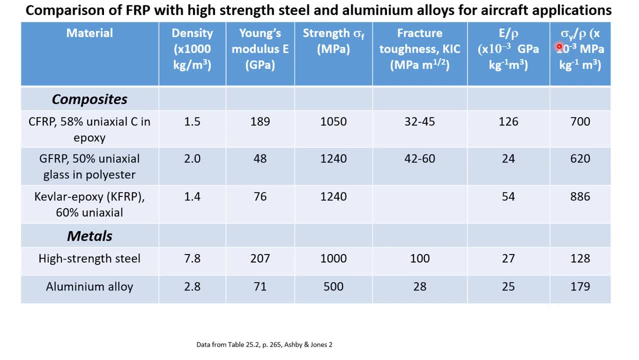 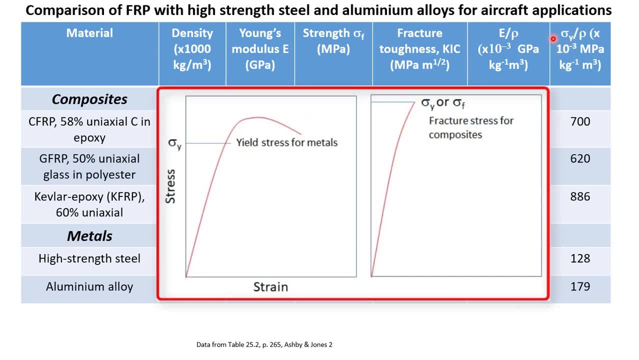 which is Sigma Y over rho. Sigma Y represents the fracture strength or the yield strength. So in the case of composites, we will use the fracture strength. in the case of metals, we will use the yield strength divided by the density. using these units. Now we can see that this ratio, again this: 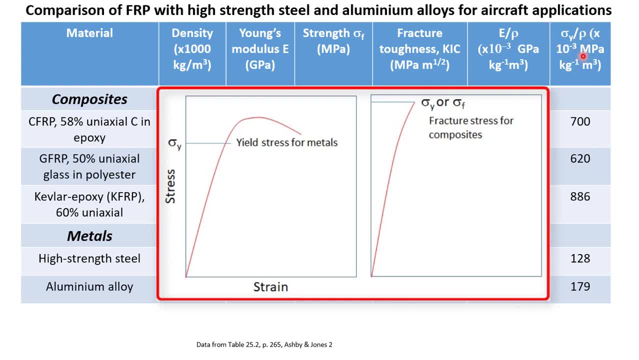 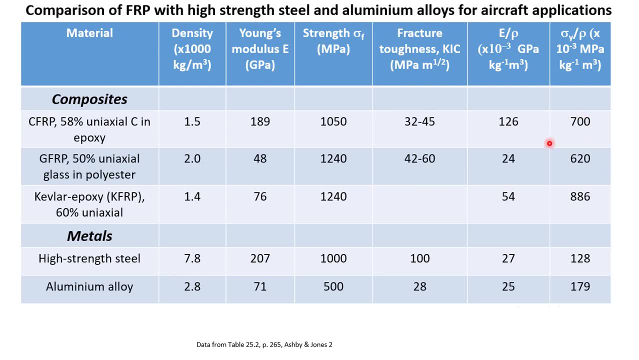 ratio represents the strength per unit density. The higher the value, the better will be strength and lighter will be the structure. So here from here we can see that CFRP has got 700, compared it with metals, which is very, very low. So CFRP will. 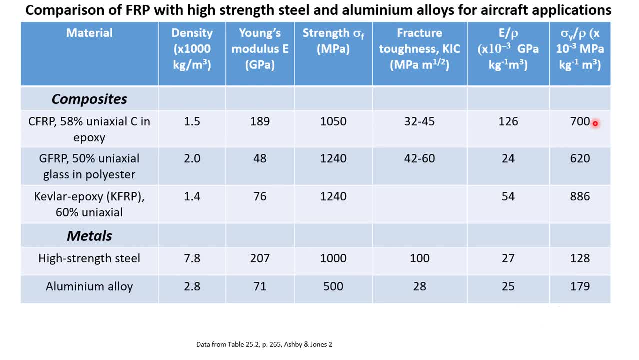 again give you very high, very strong material and very light material. Now, among these composites, Kevlar composite gives better performance: 886, 886. so that means Kevlar is much stronger and lighter compared to CFRP. So because this particular material, Kevlar, has very high strength. 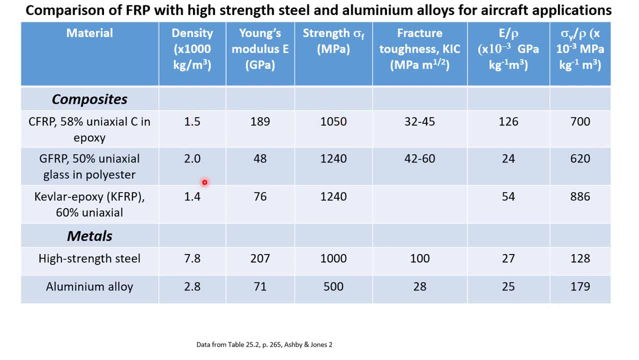 compared to carbon fiber composites. and the density of Kevlar is also low, lower than the carbon carbon fiber. so that's why we get a very high value of this ratio. For the metals, basically the density is high. for steel, density is very high. aluminium is a light metal, so density is. 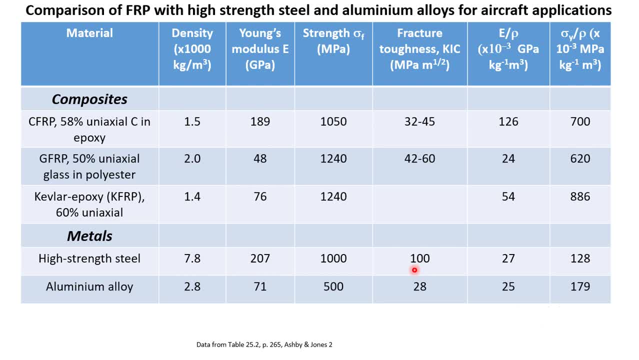 still higher than the density of these composites and in terms metal, high strength steel is very close to carbon fiber composites, but aluminum strength is quite low, so therefore we get very low values of this ratio. so now for any light weight application, we will compare these two ratios. of course we 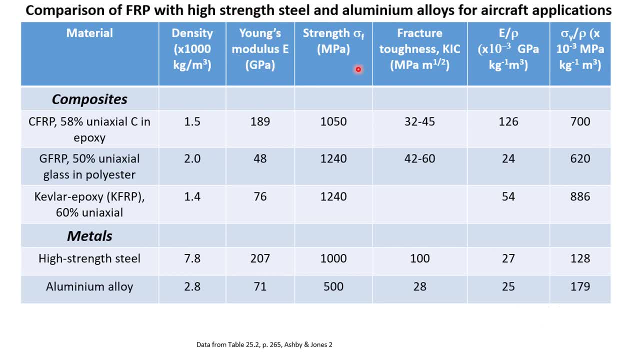 will compare the absolute values of Young's modulus strength and fracture toughness. but for our decision making, we should also compare E over Rho and Sigma Y over Rho so that we can make a decision what material will be the best for our application. so this presentation of these data basically tells us that. 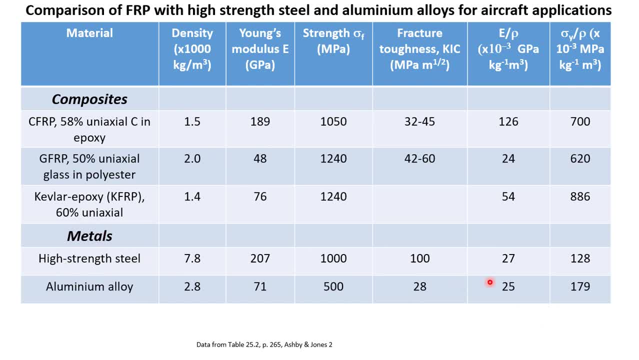 composites are better compared to metals for their stiffness and strength when they are compared in terms of per unit density. so they give us light structure but stiff and strong. so this is the reason why composites are favored compared to metals. to the metals Now, only from the stiffness and strength point of view. among the composites it 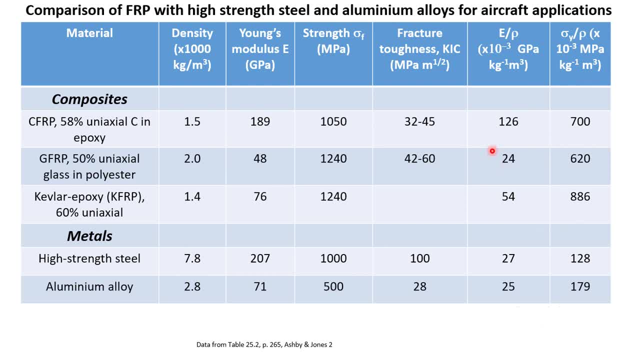 is quite sure that GFRP does not qualify for very high and very light structural applications. So we will have to restrict to CFRP, which has got very high stiffness for its density, or Kevlar fiber composite, which has got very high strength per unit of density. So our decision: 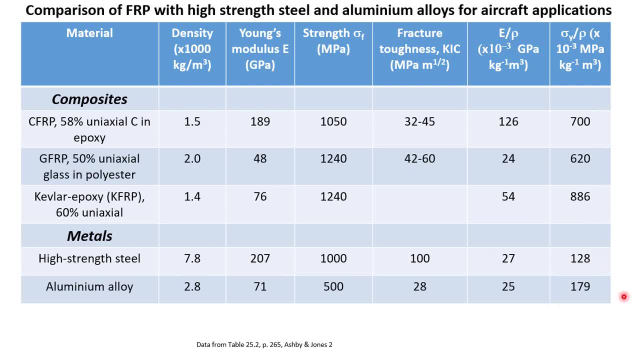 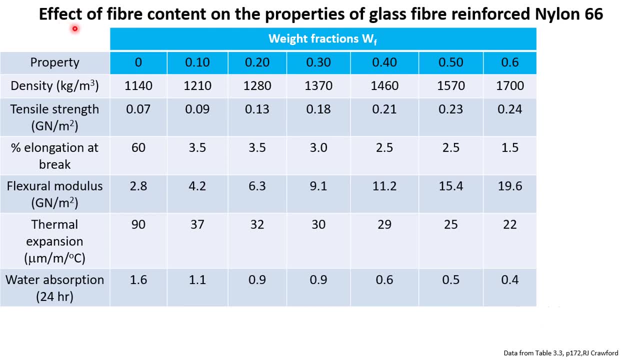 will be based on these data and whether our structure is stiffness based design or strength based design. Some more examples here: effect of fiber content on the properties of glass fiber. reinforced nylon 6-6.. So we can see that with the increasing weight fraction here we have got weight. 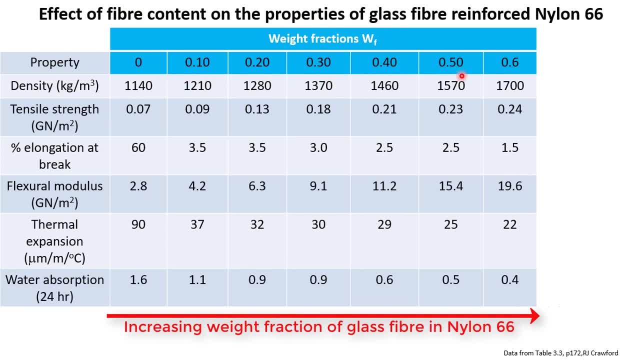 fraction, not volume fraction. So as we increase the weight fraction of glass fiber in nylon 6-6, how the properties will change, So of course the density will change. nylon 6-6 has low density and the density will increase as we increase the. 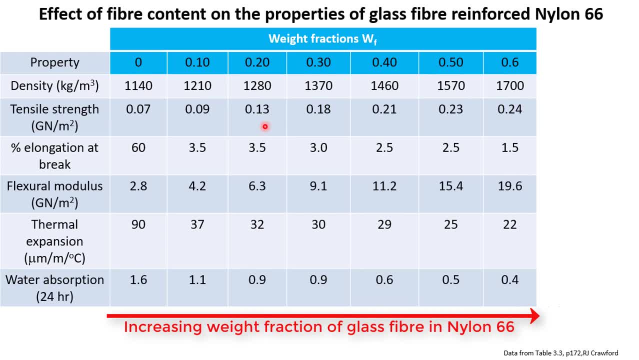 weight percentage of, or weight fraction of, glass fiber and tensile strength will also increase as we increase the weight fraction Percentage. elongation at break. this is something which tells us about the materials: toughness, how much elongation it can sustain before it fails. So nylon is a very, very tough material, so it can sustain sixty percent elongation. 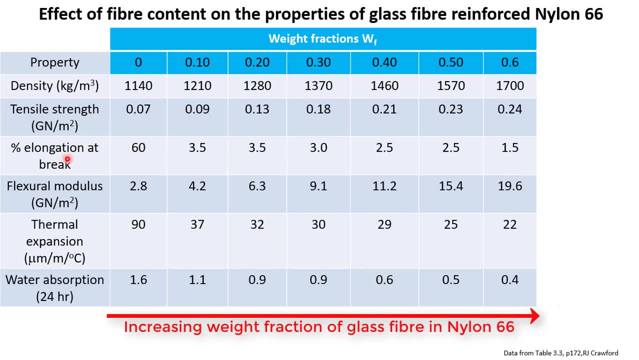 at break. but as soon as we add fiber, percentage elongation at break reduces. That means the material becomes much less ductile. So we can see that the percentage elongation at break is in the range of 3.5 to 1.5. as we increase the weight fraction of the fiber, the percentage elongation at break will. 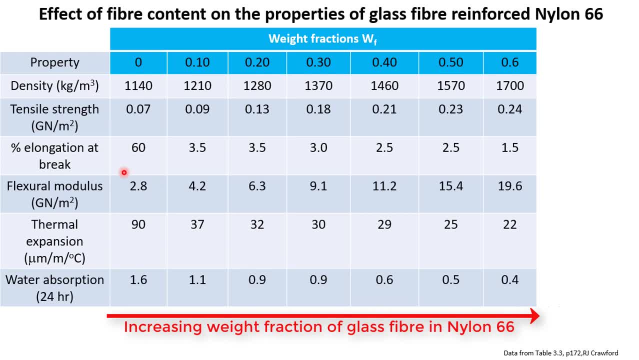 reduce Flactual modulus. it's another factor. so flexural modulus of nylon 6-6 is 2.8.. The density will increase as we increase the weight fraction. but as soon as we add glass fiber the modulus will increase to up to 19.6 for weight fraction of 0.6.. Then there are other physical 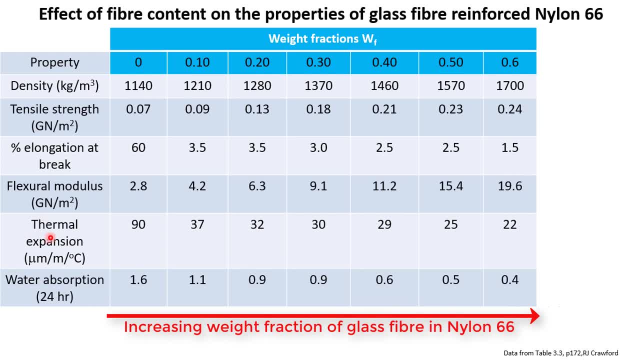 properties which are also important for composites for our mechanical design purpose, For example, thermal expansion, because the composites will be used in combination with other materials or other composites. Therefore, thermal expansion should be matched with the thermal expansion of other materials. Most of the polymers have got very high thermal expansion, but once we add fiber in it, 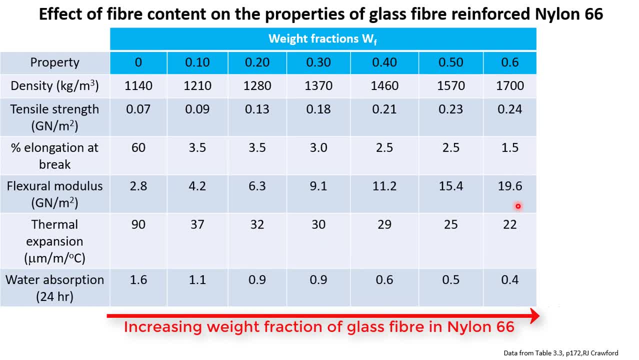 the thermal expansion will reduce, and it reduces up to 22 here in this case for 0.6 weight fraction. Now, water absorption is another property, because most of the engineering materials will be exposed to water at some point. For example, aircrafts will be exposed to rain water, and we know that polymer 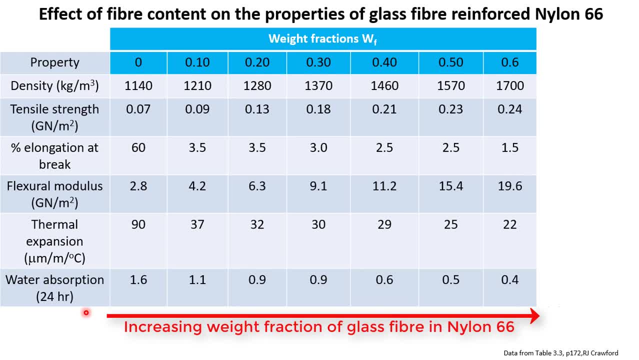 materials absorb water. As they absorb water, properties will degrade. Therefore, it is important that water absorption should be as low as possible. In the case of nylon, the water absorption is quite high. It can intake 1.6 percent of its weight in 24 hours. After adding glass fiber, the water absorption can be reduced, and it reduces to 0.4. 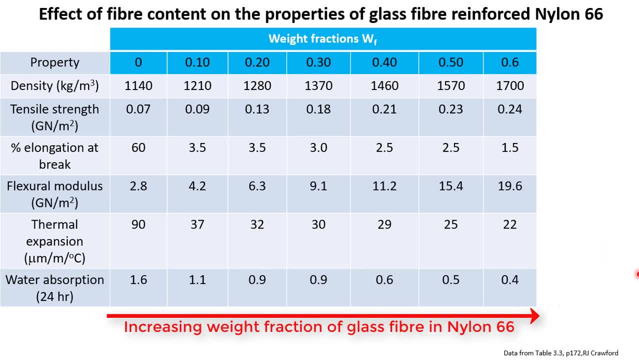 for 0.6 weight fraction. So we can see that adding glass fiber or any kind of filler material has got a very high absorption rate. So we can see that adding glass fiber or any kind of filler material has got a advantage not only in mechanical strength but also in other physical properties which are very 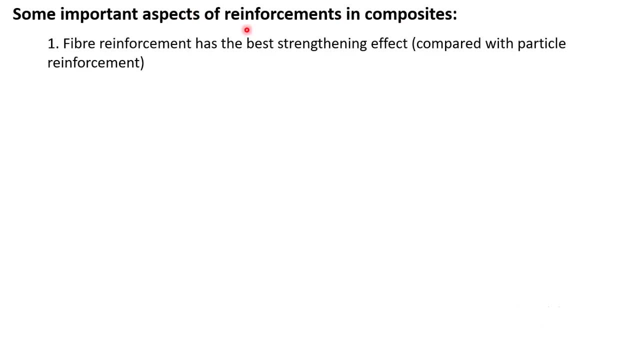 important for mechanical design. Here we will list some important aspects of reinforcements in composites. Fiber reinforcement has the best strengthening effect compared with particle reinforcement. Fiber diameter can vary from about 7 micrometer to 100 micrometer. So this is the range of fiber diameter. Fiber can be used in continuous or 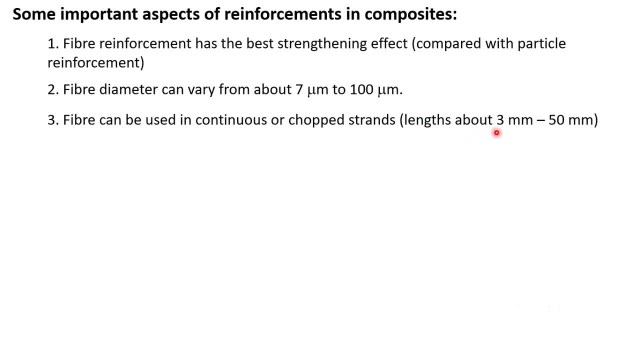 longer composites, Fiber착 is indicated with 5 sensors per aspect ratio. It can be used for części Builder para Activity Coz2 160 Ooo For chopped fiber. length to diameter ratio is known as the aspect ratio For short fiber composites, greater the 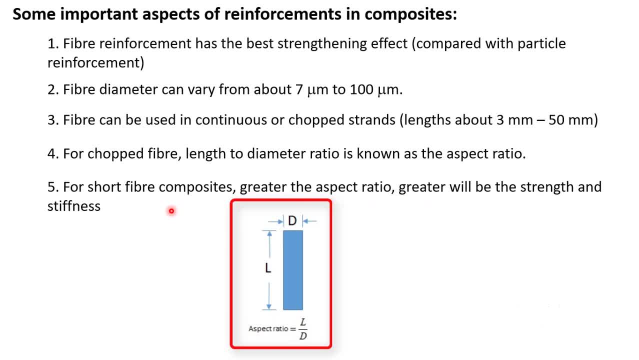 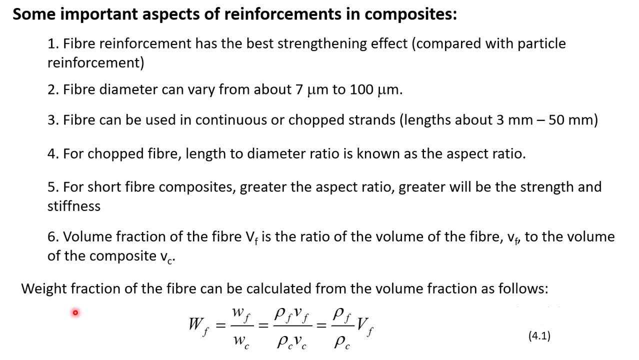 aspect ratio, greater will be the strength and stiffness. Its longer the fiber, better will be the strength effect. Volume fraction of the fiber V f is the ratio of the volume of the fabric v f to the volume of the composite. education We see many times weight fractions are given. 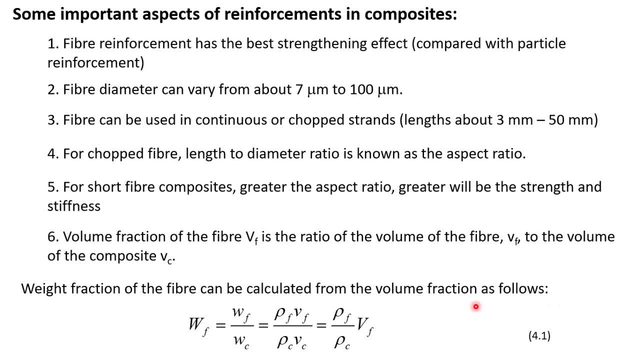 So weight fraction of the fiber can be calculated from the volume fraction as follows. So weight fraction of the fiber is equal to weight of the fiber divided by the weight of the composite, And it is given as the density of the fiber multiplied by the volume of the fiber divided. 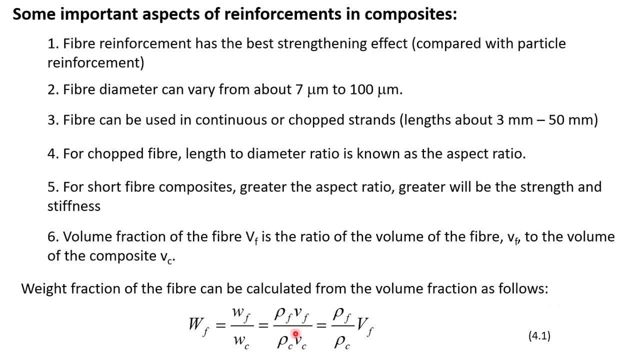 by density of the composite multiplied by the volume of the component. So finally we can write in this form: density of the fiber over density of the composite multiplied by the volume fraction of the fiber. so that will be the weight fraction of the fiber. so 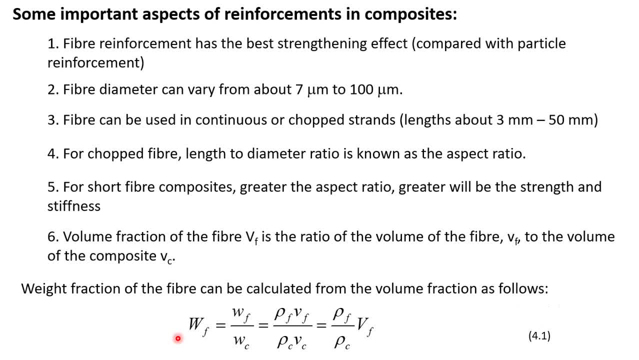 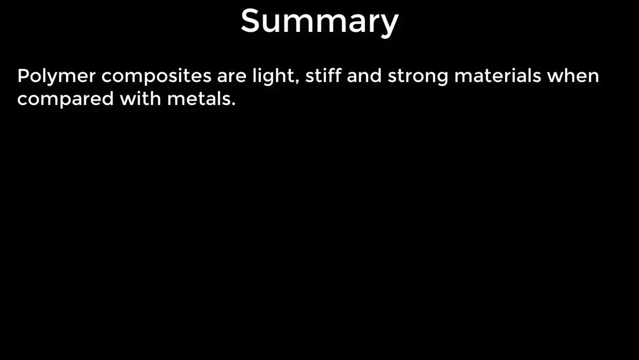 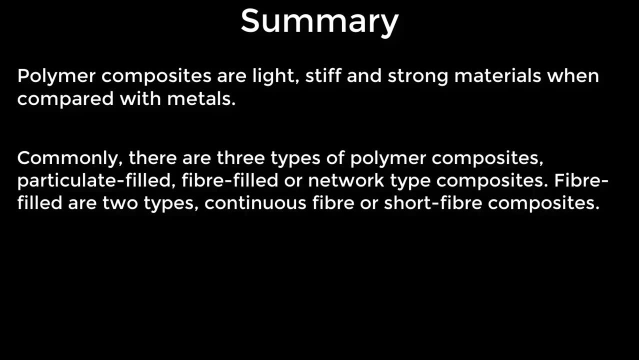 either weight fraction or volume fraction can be used for our any calculation purpose. I would like to summarize. polymer composites are light, stiff and strong materials when compared with metal. commonly, there are three types of polymer composites: particulate field, fiber field or network type composites. fiber field are two types: continuous fiber or short fiber composite. 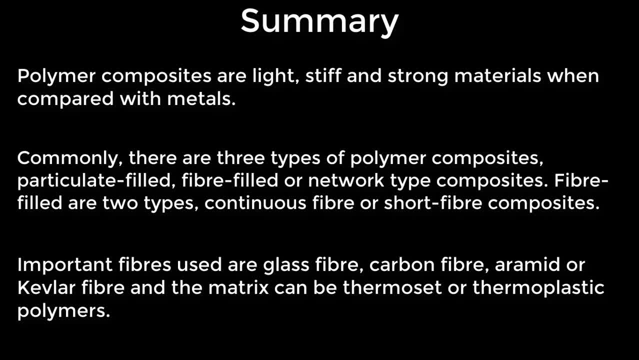 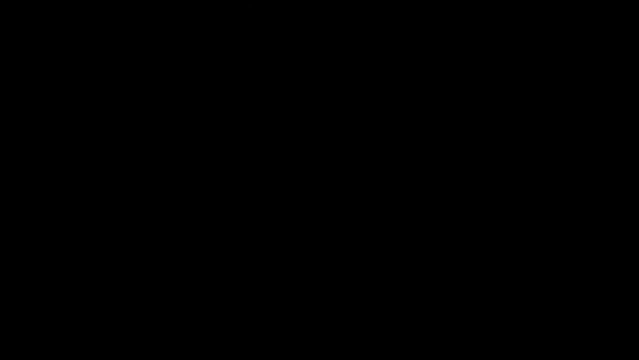 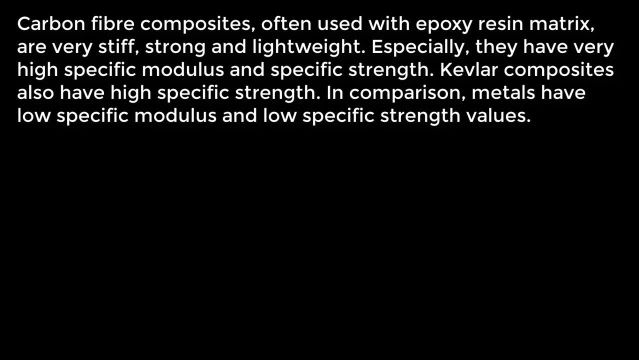 important fibers used are glass fiber, carbon fiber, aramid or Kevlar fiber, and the matrix can be thermoset or thermoplastic polymer. carbon fiber composites, often used with epoxy resin matrix, are very stiff, strong and lightweight, especially when it comes to polymer composites. 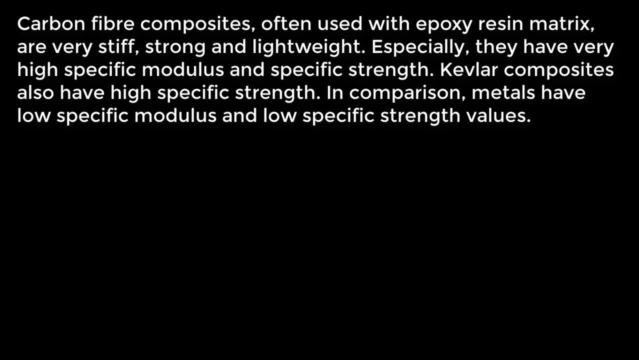 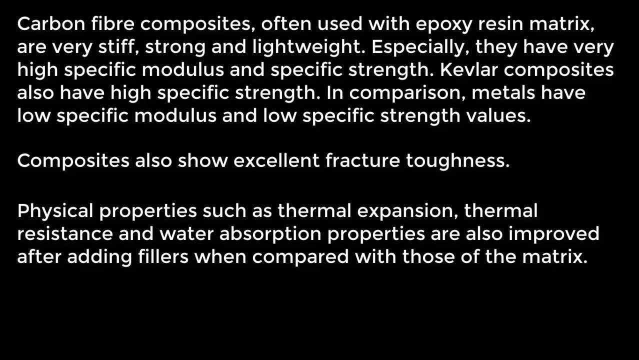 they have very high specific modulus and specific strength. Kevlar composites also have high specific strength. in comparison, metals have low specific modulus and low specific strength values. composites also show excellent fracture toughness. physical properties such as thermal expansion, thermal resistance and water absorption properties are also improved after adding fillers, when